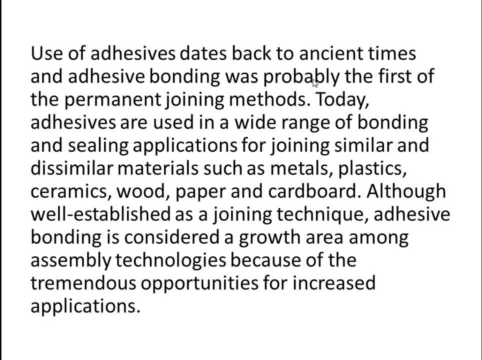 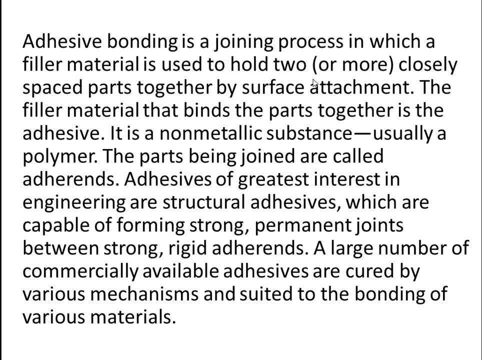 Although well established as a joining technique, adhesive bonding is considered a growth area among assembly technologies because of the tremendous opportunities for increased applications. Adhesive bonding is a joining process in which a filler material is used to hold two or more closely spaced parts together by surface attachment. 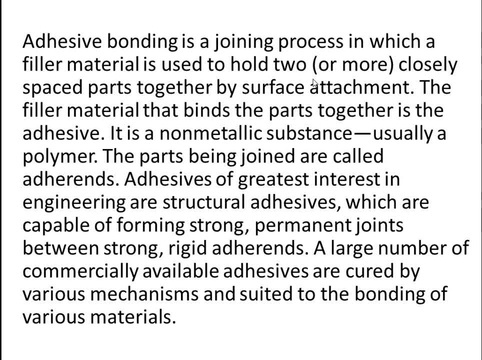 The filler material that binds the parts together is the adhesive. It is a non-metallic substance, usually a polymer. The parts are made of a non-metallic material. The parts being joined are called adherents. Adhesives of greatest interest in engineering are structural adhesives which are capable of forming strong, permanent joints between strong, rigid adherents. 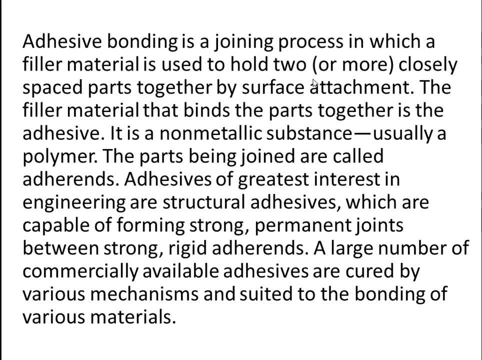 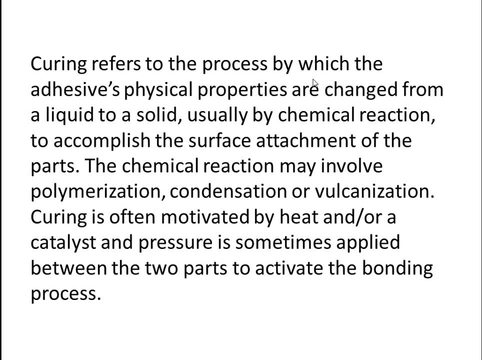 A large number of commercially available adhesives are cured by various mechanisms and suited to the bonding of various materials. Curing refers to the process by which the adhesive's physical properties are changed from a liquid to a solid, usually by chemical reaction, to accomplish the surface attachment of the parts. 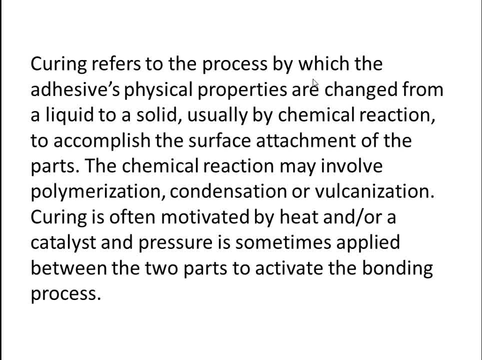 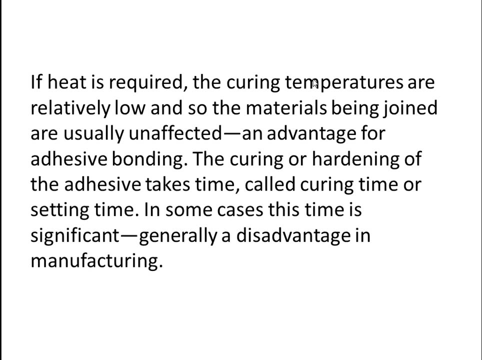 The chemical reaction may involve polymerization, condensation or vulcanization. Curing is often motivated by heat, A catalyst, and pressure is sometimes applied between the two parts to activate the bonding process. If heat is required, the curing temperatures are relatively low and certain materials being joined are usually unaffected. 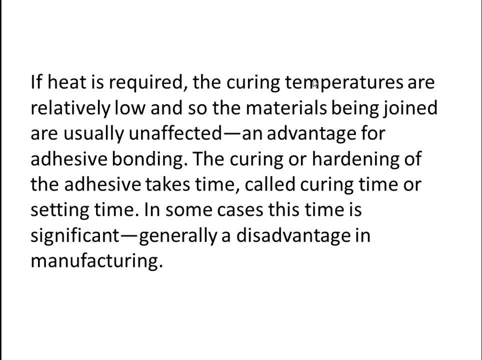 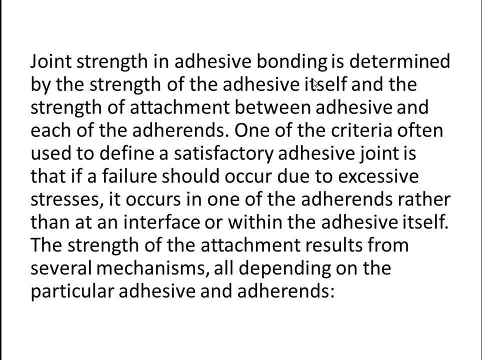 An advantage for adhesive bonding. the curing or hardening of the adhesive takes time, called curing time or setting time. In some cases this time is insignificant. Generally are disadvantages in manufacturing Joint. strength in adhesive bonding is determined by the strength of the adhesive itself and the strength of the attachment between adhesive and each of the adherents. 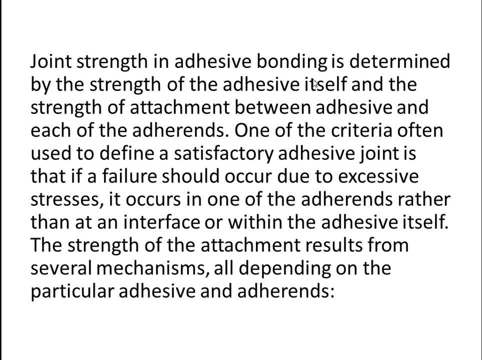 One of the criteria often used to define a satisfactory adhesive joint is that, if a failure should occur due to excessive stresses, it occurs in one of the adherents rather than at an interface or within the adhesive itself. The strength of the attachment results from several mechanisms, all depending on the particular adhesive and adherents. 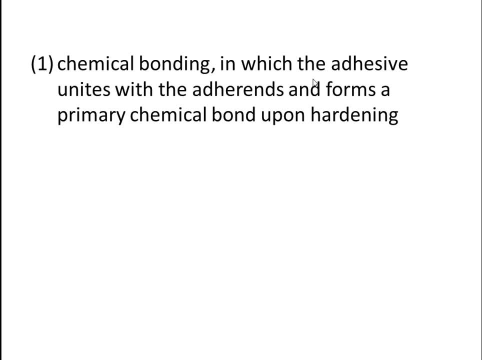 First one: Chemical Bonding, In which adhesive unites with the adherents and forms a primary chemical bond upon hardening. Second one: Physical Interactions, In which secondary bonding forces result between the atoms of the opposing surfaces. Third one: Mechanical Interlocking. 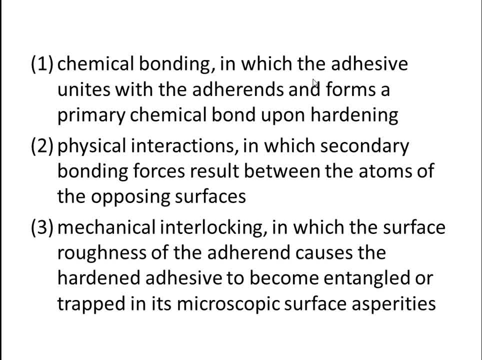 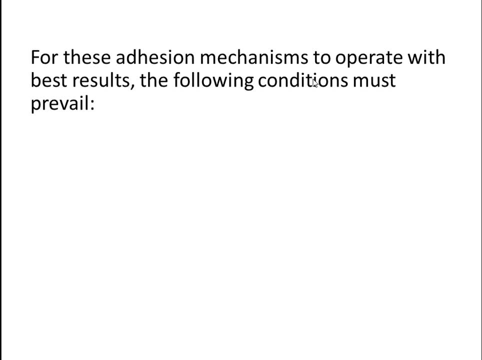 In which the surface roughness of the adherent causes the hardening of the adhesive. The hardening of the adhesive causes the hardening of the adhesive to become entangled or trapped in its microscopic surface activities. For these adhesion mechanisms to operate with best results, the following conditions must prevail: 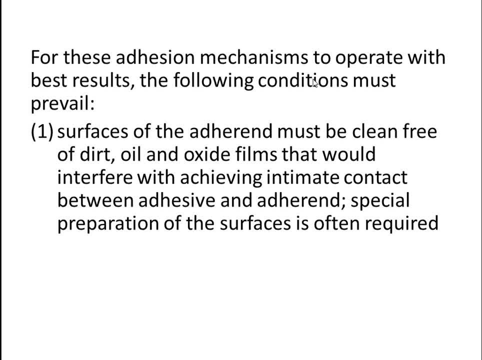 First condition is Surfaces of the adherent must be clean, free of dirt, oil and oxide films that would interfere with the adhesion. With achieving intimate contact between adhesive and adherent, Special preparation of the surface is often required. The adhesive in its initial liquid form must achieve thorough wetting of the adherent surface. 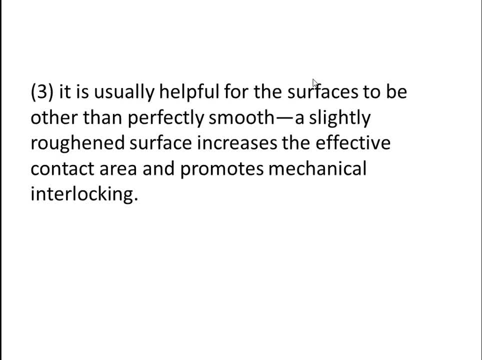 Third one: It is usually helpful for the surfaces to be other than perfectly smooth. A slightly roughened surface increases the effective contact area and promotes mechanical interlocking. In addition, the joint must be designed to exploit the particular strength and adhesive bonding and avoid its limitations. 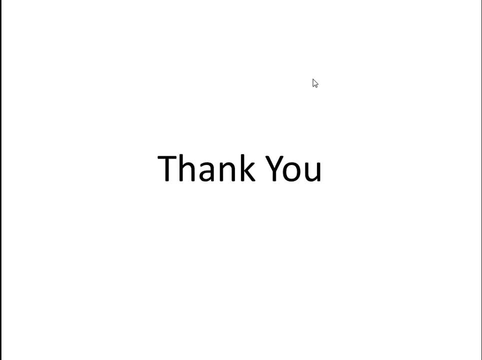 And finally, thank you for being with me.